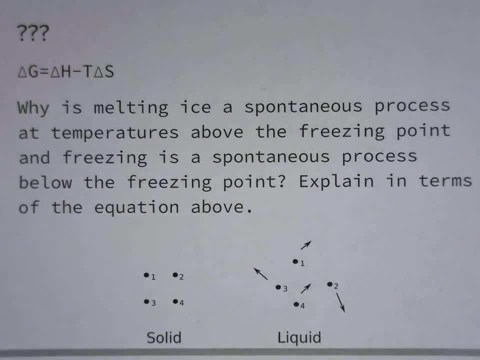 Let's consider this question: Why is melting ice a spontaneous process at temperatures above the freezing point and freezing is a spontaneous process below the freezing point? Explain in terms of the equation above. So let's illustrate what happens when we're melting something and freezing. 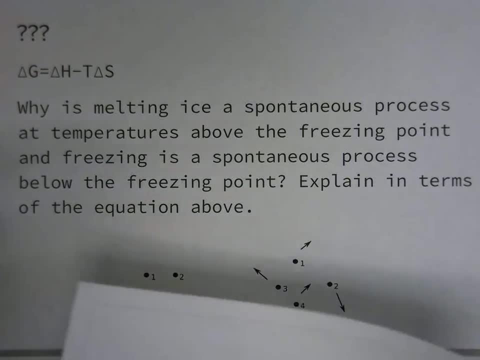 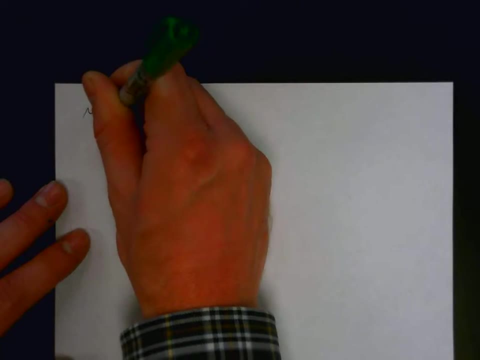 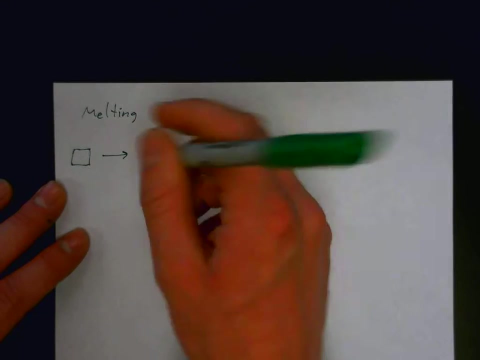 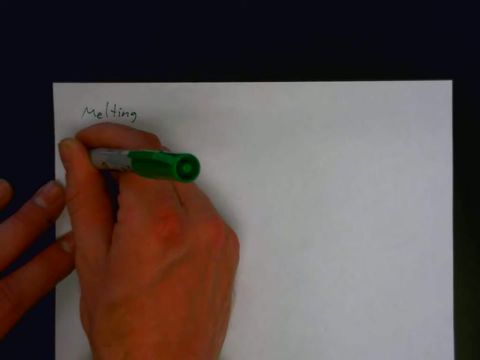 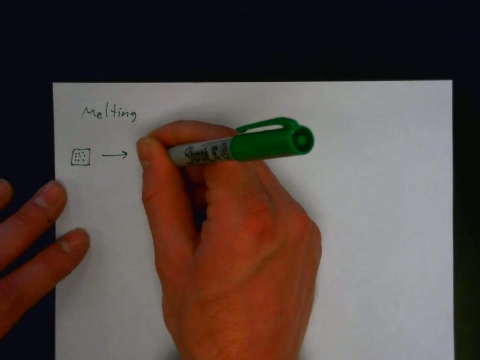 You can see illustrations of the solid and the liquid form. So during the process of melting we have a solid becoming a liquid. Now the entropy of a solid is less than the entropy of a liquid. So in a liquid the particles have more motion. 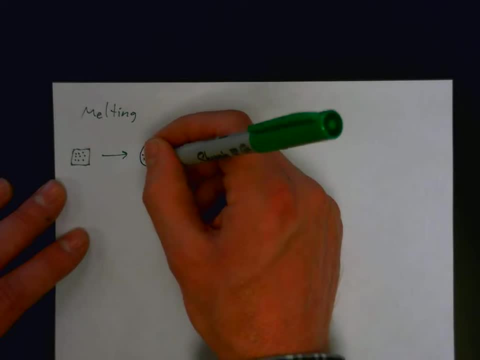 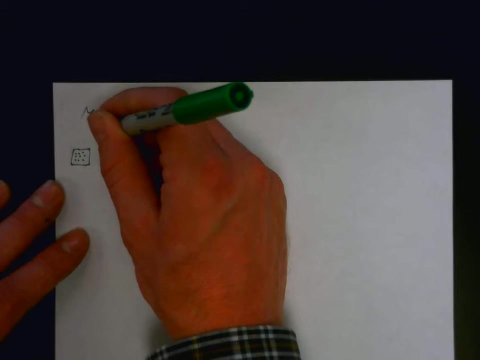 There's a higher probability that they will be in the liquid. the additional motion of the liquid state, higher entropy in this state versus the solid state. Or we could say there's more disorder in the liquid state. So as we go from a solid to a liquid, the entropy is increasing. 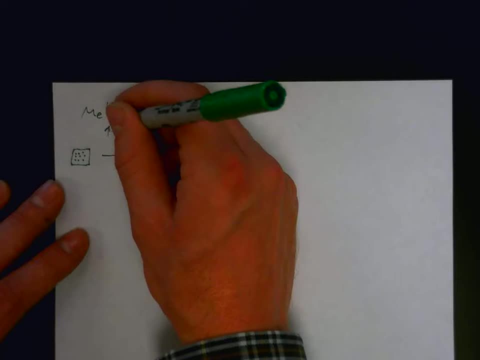 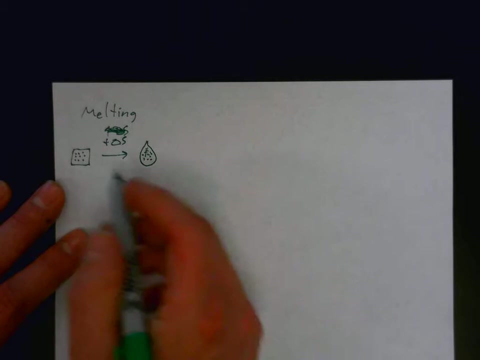 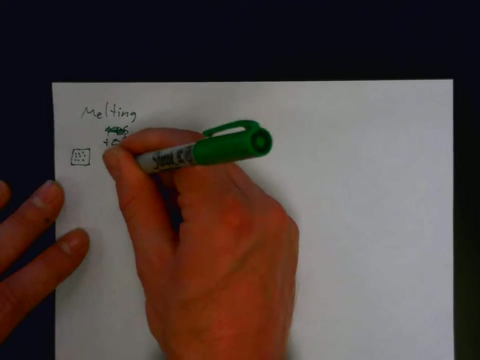 So delta S is positive. So we have a positive delta S. Let me rewrite that: So positive delta S Now, as we go from the solid to a liquid state, is the enthalpy delta H. would that be increasing or decreasing? 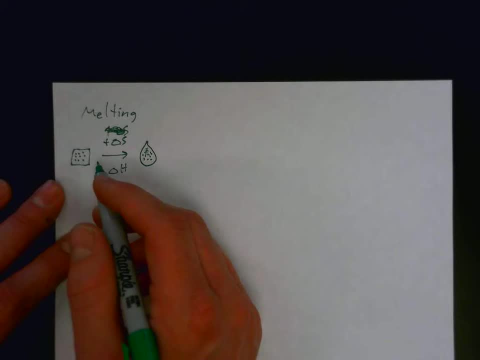 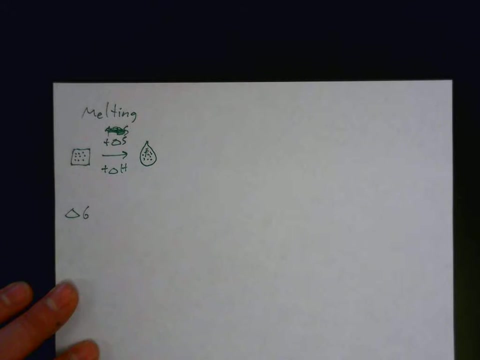 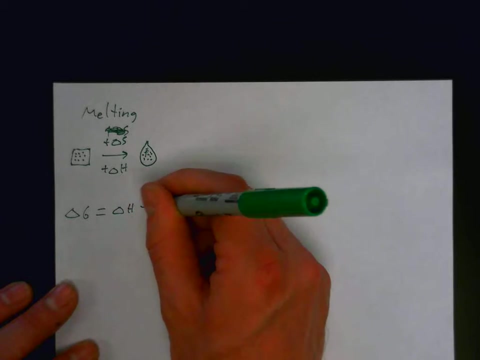 So delta H would be also positive. This is an endothermic process. We have to add heat in order to melt ice. So let's think about the equation. The delta G value is the enthalpy minus the temperature times the change in entropy. 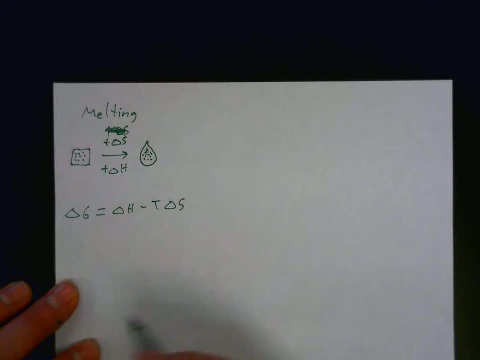 So the, The change in enthalpy is positive And the change in entropy is also positive. However, as a term for this whole term notice- we have a negative sign. So this whole term, if the entropy is positive, that gets multiplied by a negative. 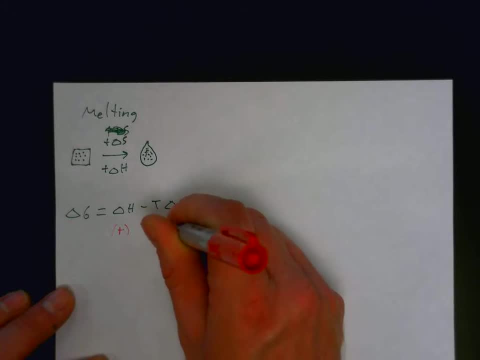 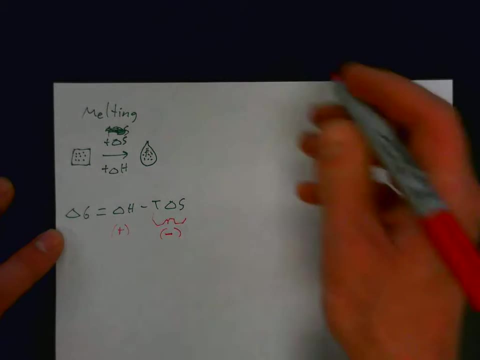 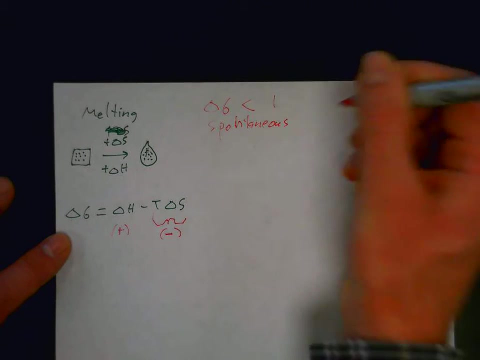 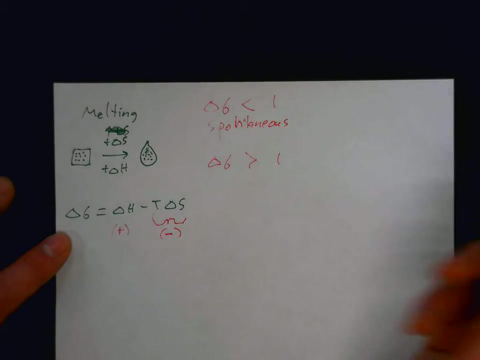 which means that the whole term would be negative. Now we know that the process is spontaneous if delta G is negative. So if delta G is less than 1, that's spontaneous, So that's spontaneous. And then if delta G is greater than 1, that would be non-spontaneous. 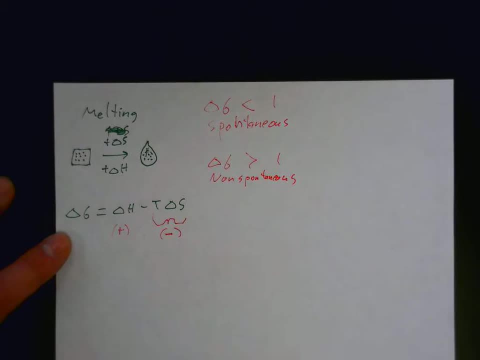 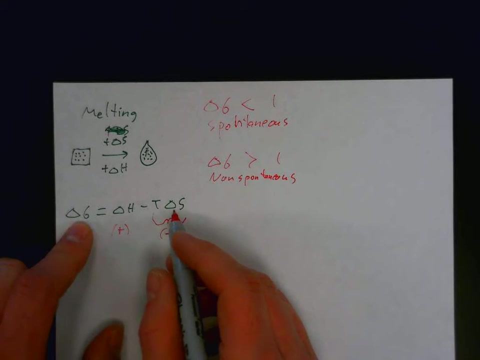 And then when delta G is equal to 1, that is equilibrium. So now it comes down to a balance of how much the temperature affects this situation In order for delta G to be negative. the entropy, this term, the entropy times, the temperature. 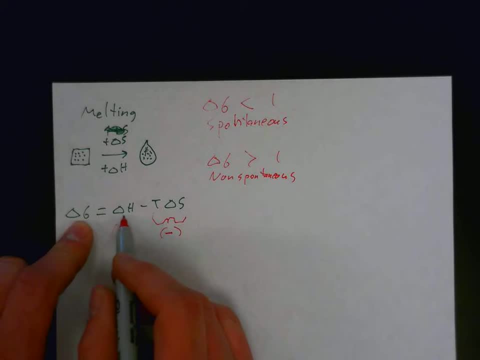 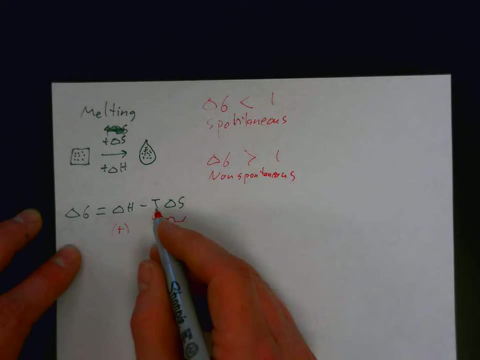 has to amount to a greater value than the temperature. So this is the temperature, So the temperature is higher than the enthalpy, So that the overall value for delta G comes out as negative. So the thing that affects this, then it comes down to the value of T. So when the temperature is high, this term is higher, a greater value than the enthalpy, resulting in an overall negative delta G value, And it supports our common sense That melting happens at higher temperatures. So let's illustrate, then, what happens during freezing. 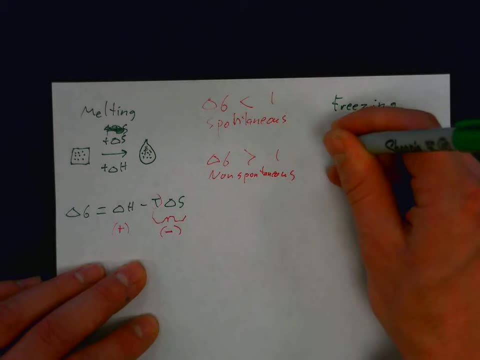 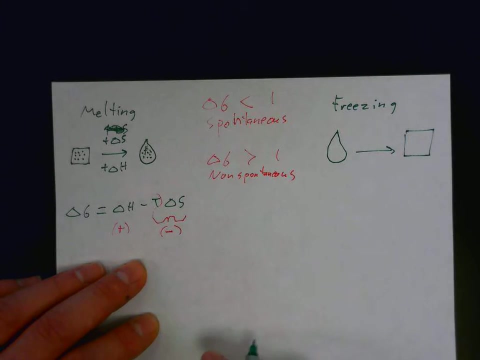 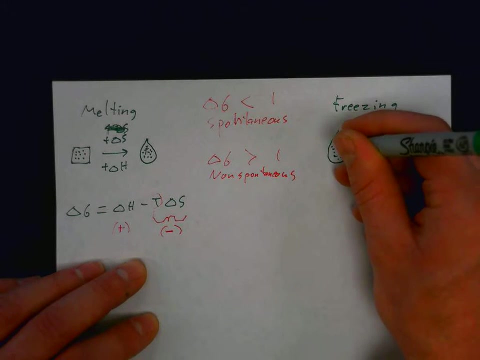 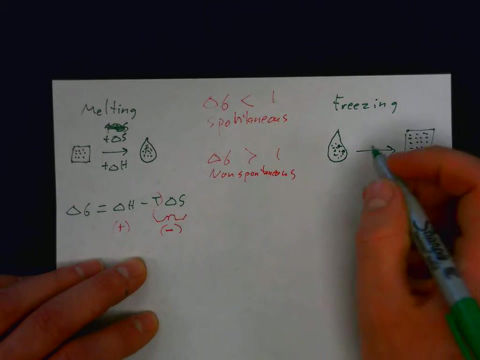 So freezing is when a liquid becomes a solid, So the entropy is higher in the liquid state- It's a more disordered form, we could say, Than the solid state. So the entropy as it goes from a liquid to a solid is decreasing.